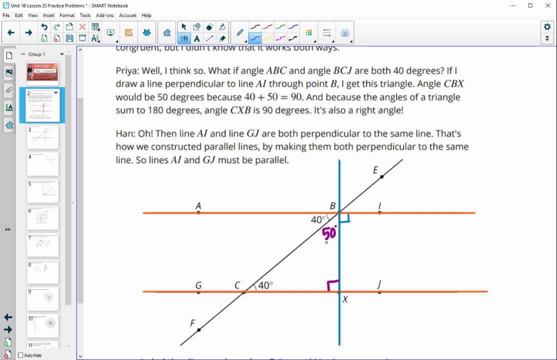 Okay, So we know then that this one is 90, because 40 plus 50 plus 90 would be the 180 degrees. So then that means that CXB is 90 degrees. So it's also a right triangle. So she made this. 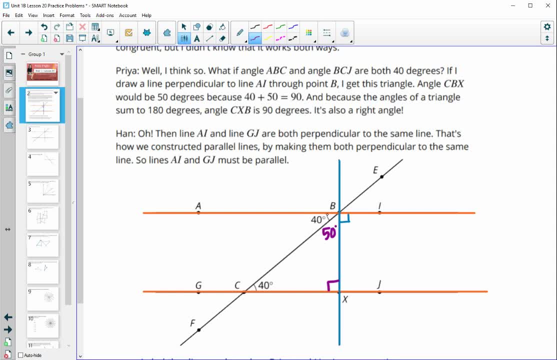 line perpendicular here, figured out that this was 50 by this being a straight line. Then did 180 minus 50 minus 40 to get that this one is 90 also. So then Han says, oh a line, AI and GJ are then. so these orange lines are both perpendicular to the same line. 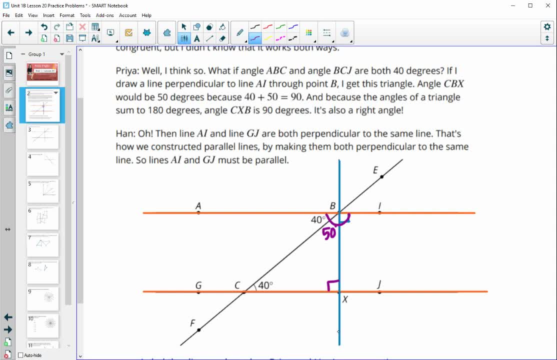 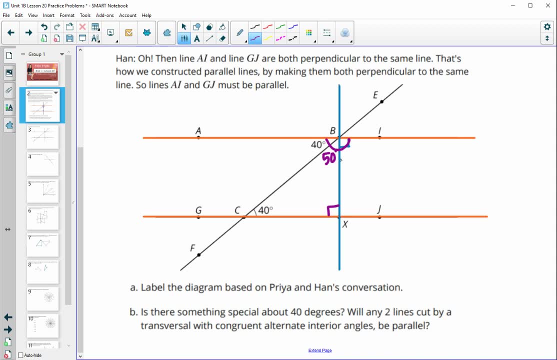 the blue one. That's how we constructed parallel lines, by making them both perpendicular to the same lines. So AI and GJ must be parallel, So label the diagram, which is what we did, Based on their conversation. and was there anything special about the 40 degrees? Okay, 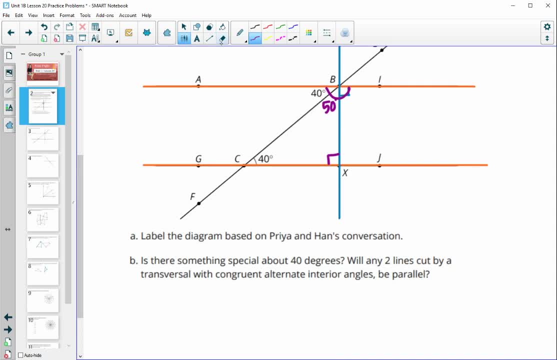 Or basically, could we change that? Could we have had that be a different number? So if I delete this and if we just changed this number, like if these were both 20, then we could do 180 minus 90 minus 20 and get 70 here, And then, when we do 180, minus 70 minus 20, we would get 90.. 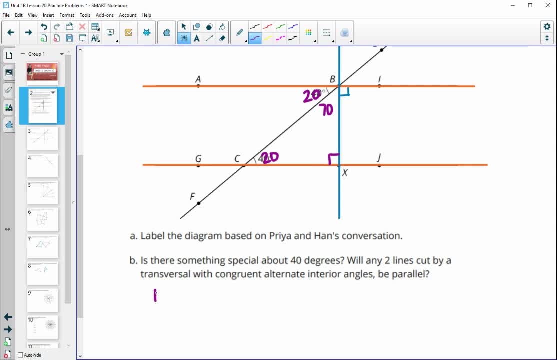 So there was nothing. So is there anything special about the 40 degrees? No, this will work for any angles, So for any alternate interior angles that are congruent, Which we're going to look at now in number two, because number two says so, prove it. 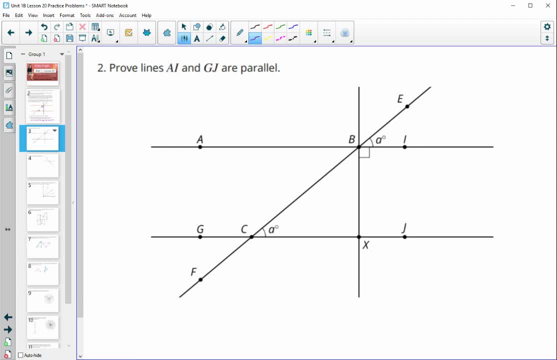 OK, which proving it means that we're not going to use any specific numbers, So that it'll work for anything. So in this one, so prove. lines A, I and G, J are parallel. We don't have alternate interior angles here, but we can do a similar idea. 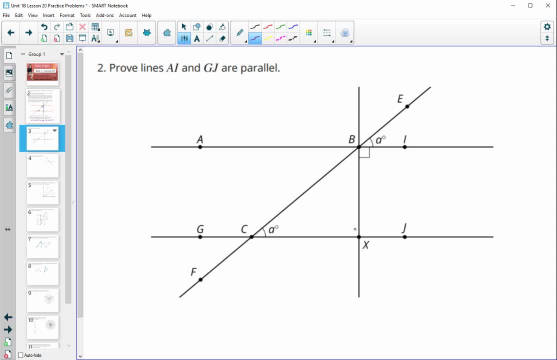 So we see that we've got this line perpendicular here. So if we could prove that this was a 90 degree angle, then we would know that the two lines- OK, this line and this line- would be perpendicular to The same line, this one. 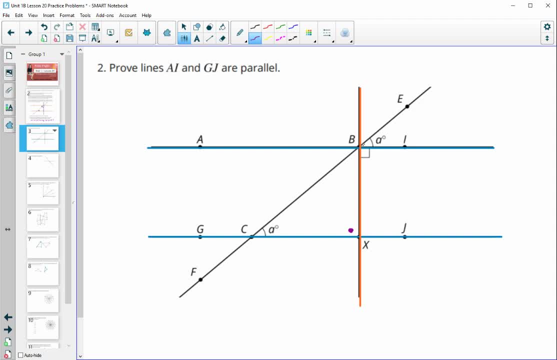 So if we're looking here, we see a straight line here With a 90 and this angle. so this angle right here, and I'm just going to write number one next to it. Just, this is my first step that I'm doing. 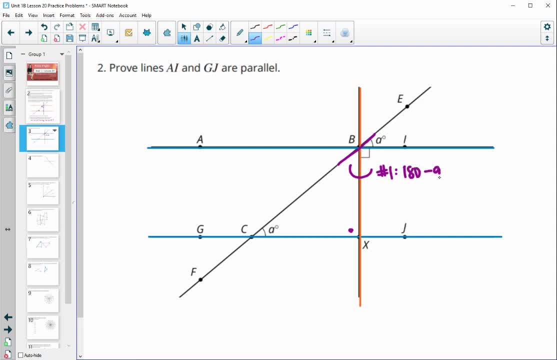 So I have a straight line. so I could do 180 and I could subtract off 90 and A to figure out that angle. So 180 minus 90 is 90. And then we still have that minus A. So this angle right here is equal to 90 minus A degrees. 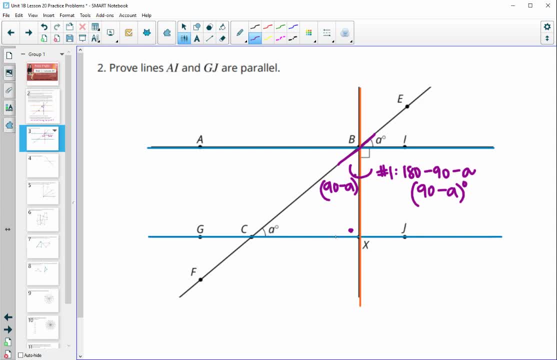 Then the second thing that I'm going to look at is this triangle, And we know that the sum of a triangle. So I'm just going to write number two next to here. We know that all the angles in a triangle add to 180.. 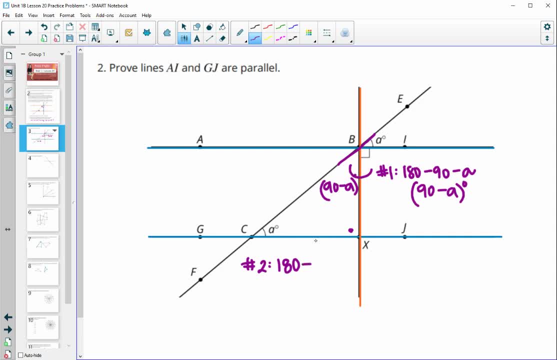 So I'm just going to subtract off the two angles that I know which is A, And then also I'm going to subtract off 90 minus A And I'm going to put parentheses. I'm going to put the parentheses in there because I'm subtracting the whole angle. 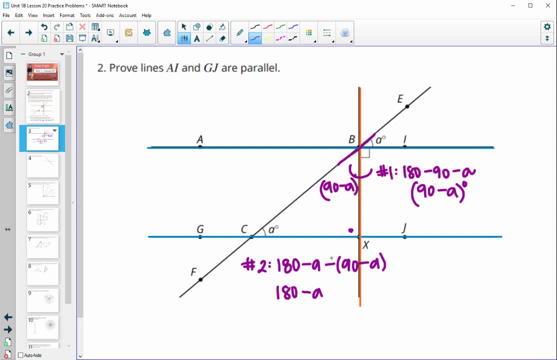 So then we'll do 180 minus A and then I'm going to bring this negative in. So we're minusing 90 and minusing a negative A which is really plus A. So I see a negative A and a positive A. that will cancel. 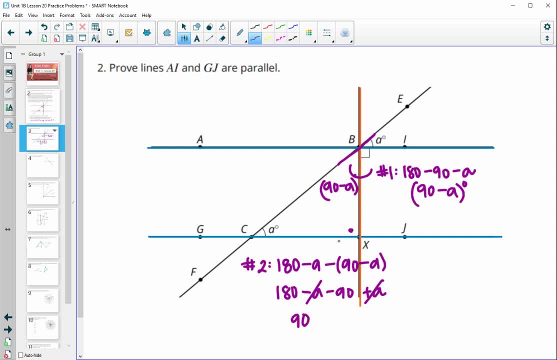 And then 180 minus 90 is 90. So that angle right there is 90 degrees, no matter what the measure of A is. So therefore, since AB and GX are both perpendicular to BX, the orange line, they are parallel to each other. 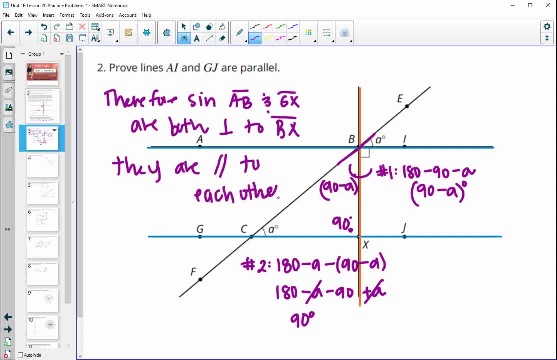 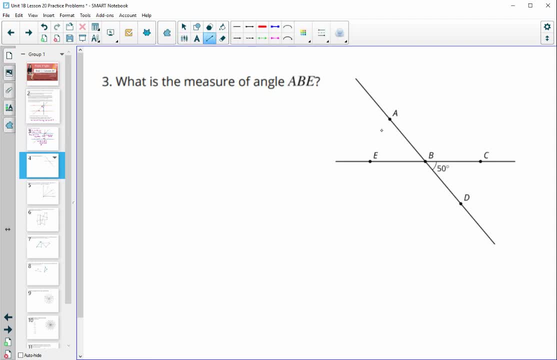 Number three: what's the measure of angle? ABE? So if you have a hard time trying to figure out what angle they're talking about, think about tracing it, So A to B to E, and then that'll show you. So just kind of follow it with your pen. 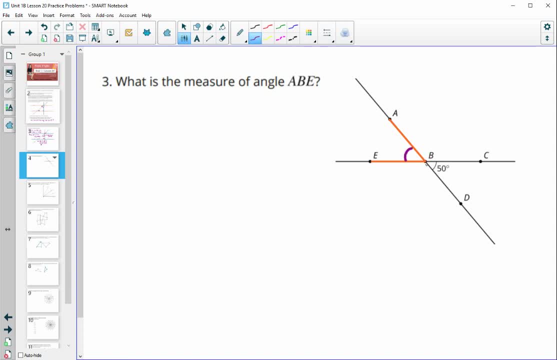 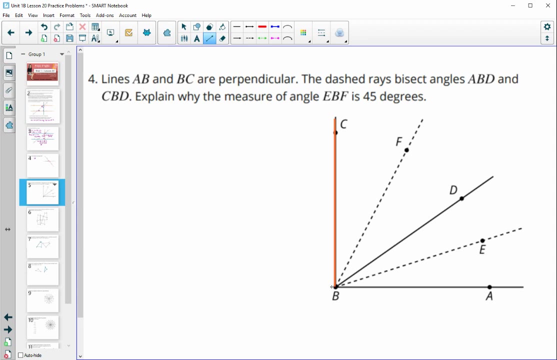 So ABE is this angle here. That's a vertical angle with this one, And vertical angles are equal to each other, So 50 degrees. Number four: lines AB and BC are perpendicular, So this one is perpendicular to this one, meaning that that forms a 90 degree angle. 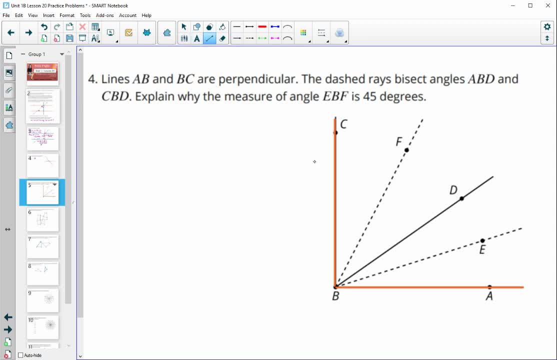 The dashed rays are the angle bisectors of these two angles, So this one bisects this angle. This one bisects this angle. Explain why the measure of angle F, EBF. so EBF is this angle, So the angle formed by the angle bisectors. 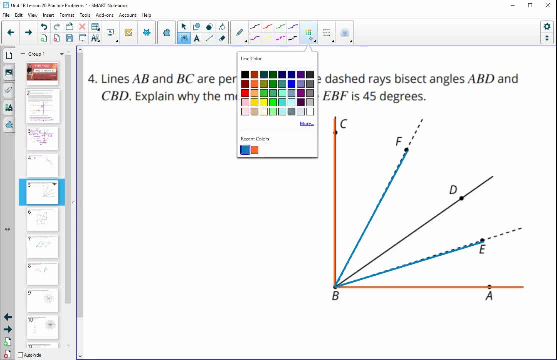 Why is that one always going to be 45 degrees, Okay? so how do we know? that is what we're looking at here. So let's look at it in general terms, because if we put numbers in here, then that's only proving it for one case. 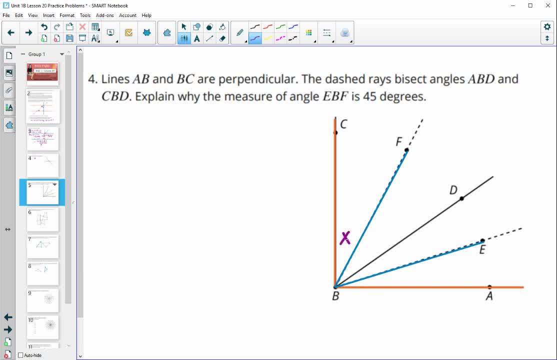 So we do know that this is an angle bisector, So I know that this angle is the same as this angle, So I'm just going to call them both X. Then, similarly, in here, we know that these two angles are equal, Not to these ones, so pick a different variable. 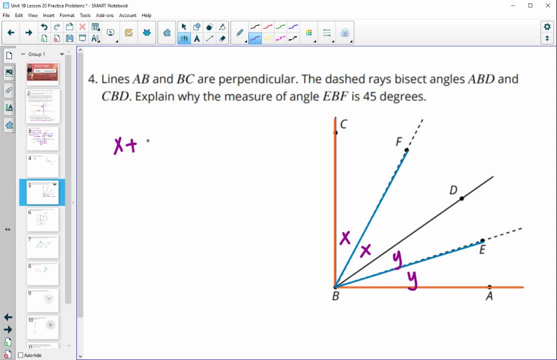 So I'm going to go with Y, And what we know is when we do, when we add all four of these little angles together, they make up that big angle which is 90 degrees. So we have two X's and we have two Y's and they equal 90.. 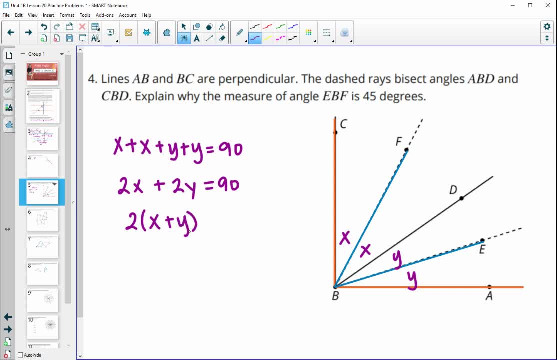 So if I distribute out a two, so I take a divisor, write a two out of each of those. we could write it like this, And then we could divide each side by two, which gets us that X plus Y is equal to 45.. 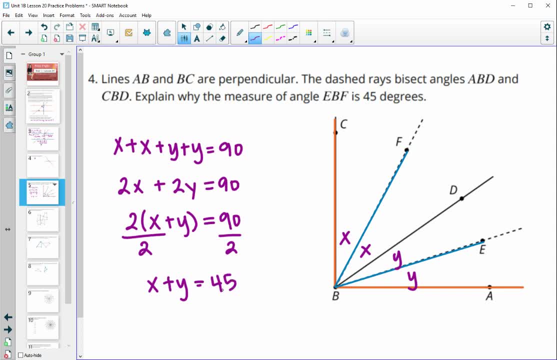 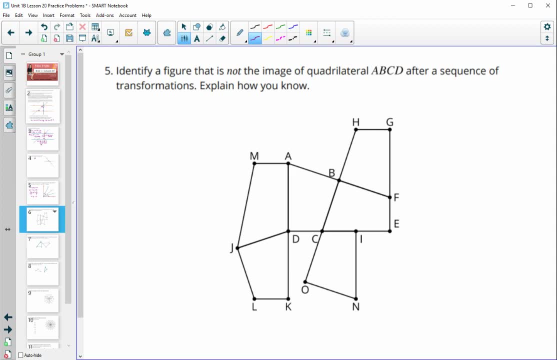 So, no matter what the angles were, okay, they will add up to 45 degrees. Number five: identify a figure that is not the image of quadrilateral ABCD. So here's ABCD. So we want to find an image or a figure in here that is not the image of this. okay, 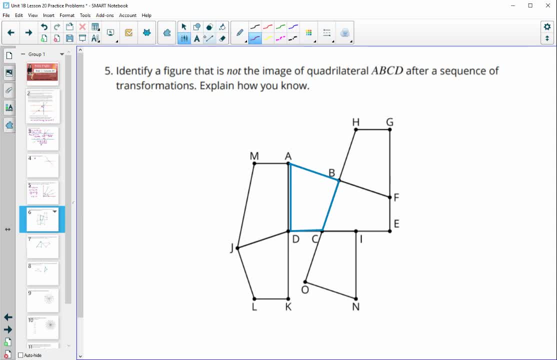 meaning from a sequence of transformations, meaning it's not the same size. So look for one that looks like it's not the same size. okay, and that would be this one right here. And we know this because if we look in ABCD, AD is the longest kind of side here. 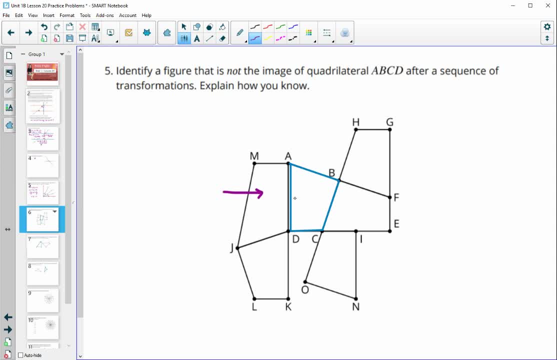 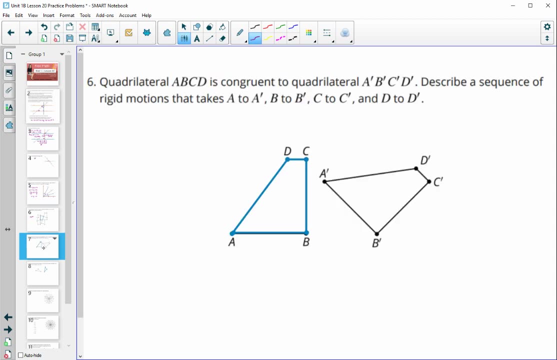 and that's not really matching okay When we go down. this MJ is elongated, so way longer than this one, And so these are not congruent. So ADJM Number six, quadrilateral ABCD, is congruent to quadrilateral A, prime B, prime C, prime D prime. 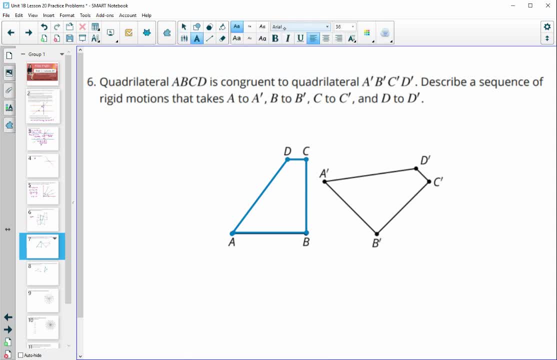 Describe a sequence of rigid motions that takes all of them onto each other. So let me type this one out here. All right, so these are not touching, So we're going to do a translation to get them touching. So translate: quadrilateral ABCD by directed line segment, whatever you want. 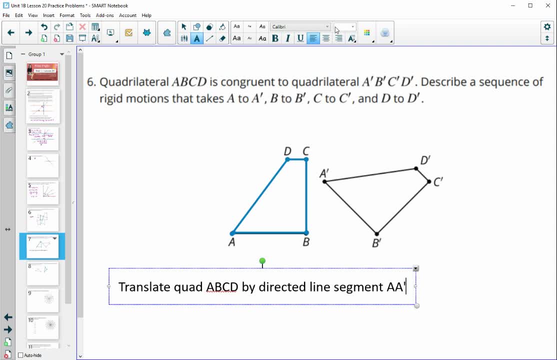 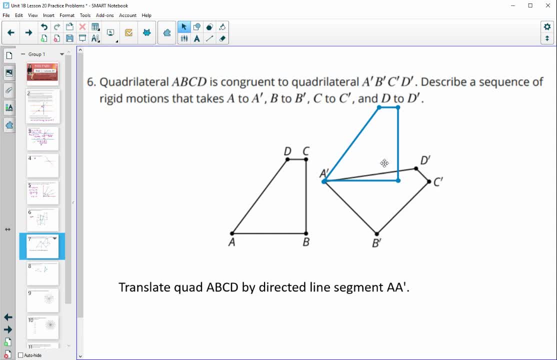 And then I'm going to rotate and we see that when we rotate B down to B prime, everything else will fall in line. So the final thing that we'll do is rotate around point A prime. So that's the fixed point, That's the point that's going to stay until- and actually we should put the figure- 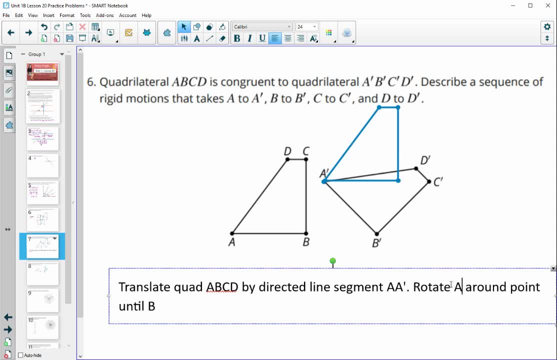 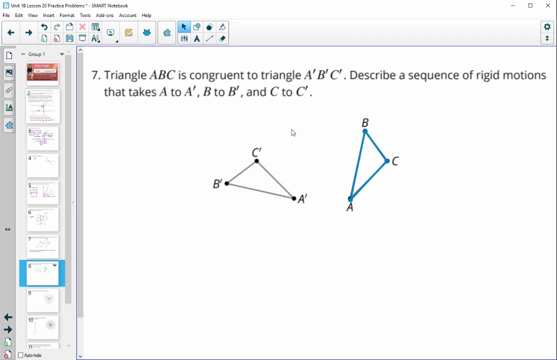 So rotate A, B, C, D around point A until B coincides with B. prime Number seven is the same thing. So taking and doing another sequence of motions here. So these are not touching. So again we'll translate to start. 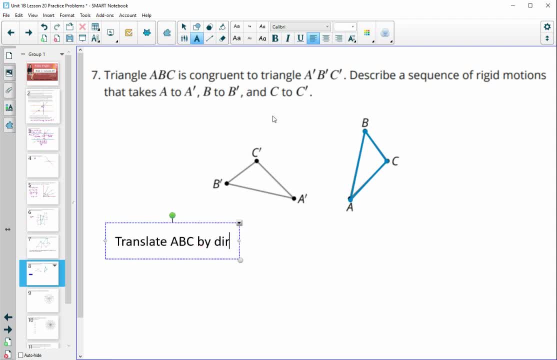 So translate A, B, C by directed line, segment A, A, prime, And this will just move the figures so that their A coincides with A prime. Now we're going to want to rotate And again you can see. so here's B.